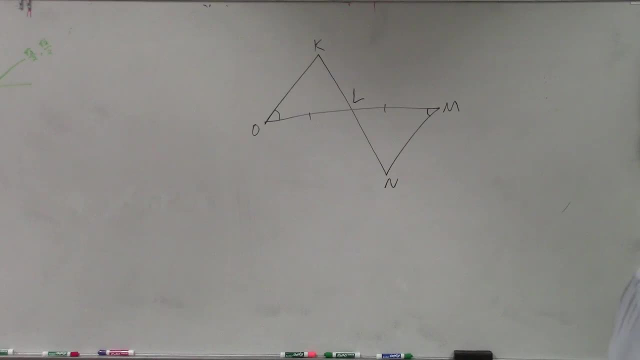 When you guys are looking at this problem, and this is number 13,. what we're trying to do in this problem is again, actually we're just trying to fill it in, but it already says proving angle k is congruent to angle n because congruent parts. 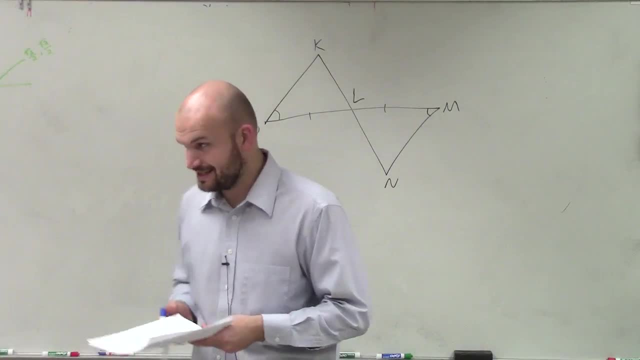 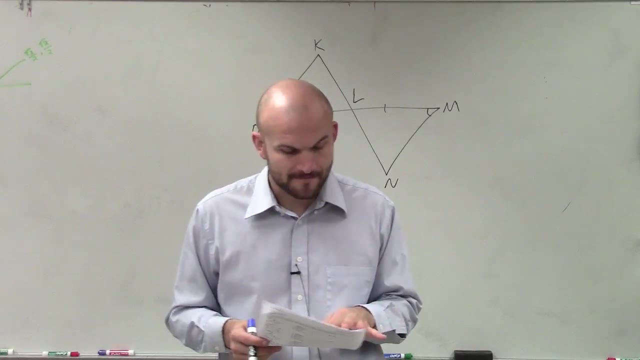 of congruent triangles are congruent. So CPCTC, that's what that means: Congruent parts of congruent triangles are congruent, And so what they're saying is: we have these two triangles, We know what we need to do to prove congruent part. 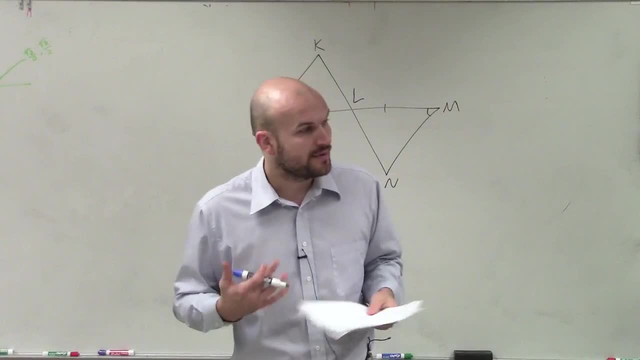 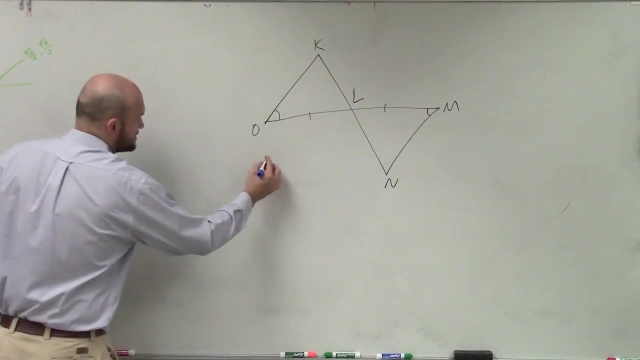 or corresponding parts- I'm sorry- of congruent triangles are congruent. We have to prove the two triangles are congruent. So when we look at this, the first thing, if I'm going to set this up again, let's first just write down what is the information that we 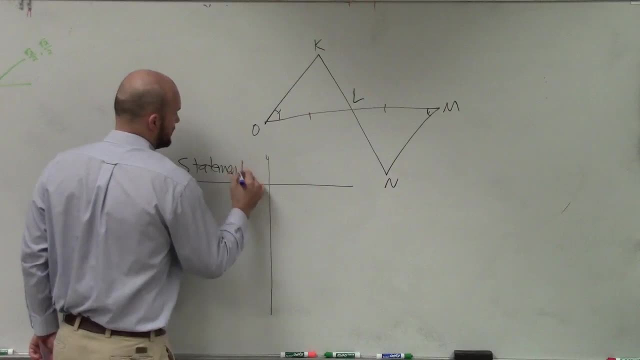 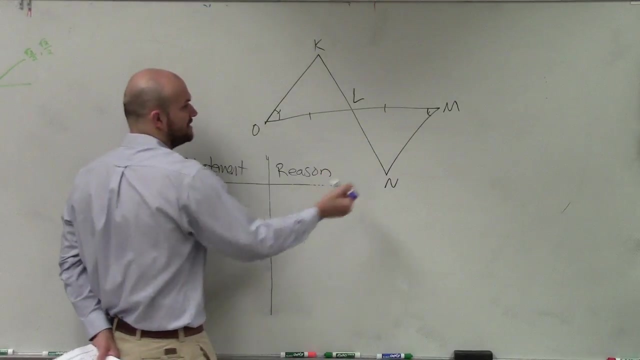 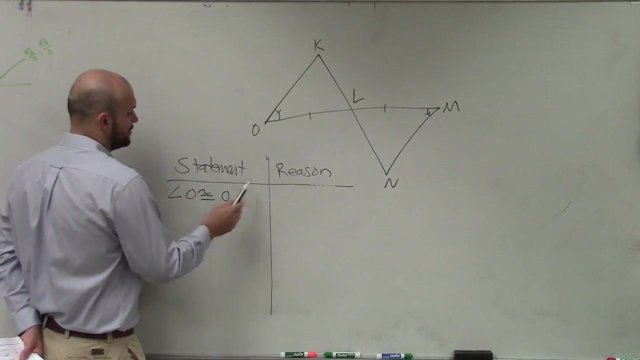 know. So we again write our statement and our reason. So again, let's just look at this. We see that these angles in this picture are given to us as equal. So I can say: Angle o is congruent to angle m, because that is given. 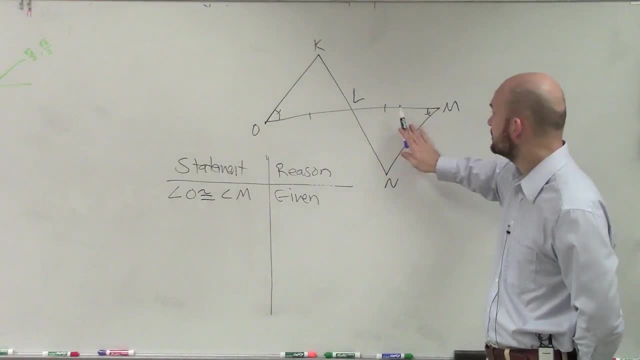 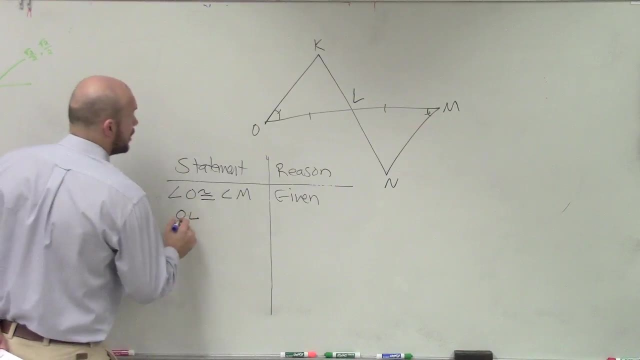 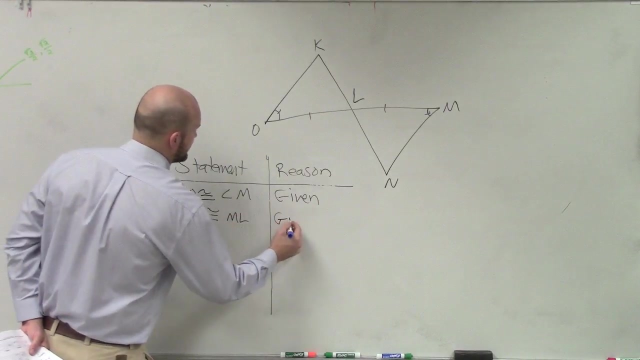 Then the next thing is we can see that this line is congruent to that line because they both have a tick mark, So they know they're equal in measure. So I can say the line ol is congruent to the line ml because that's given. 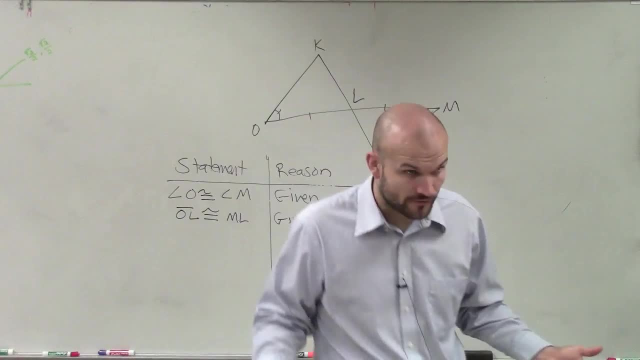 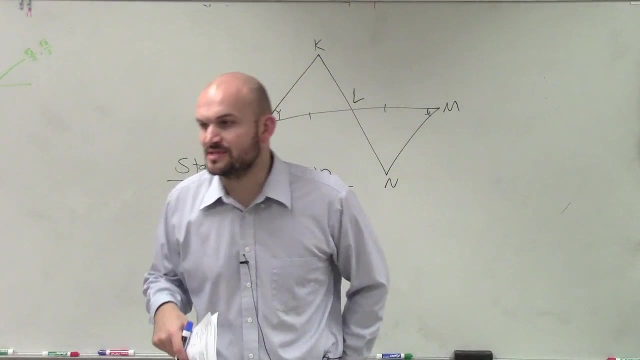 So either the givens are either going to be written out for you or they're going to be provided in your figure. Now the next thing, Zeth. I don't want to have to talk to Ms Magloff about this. 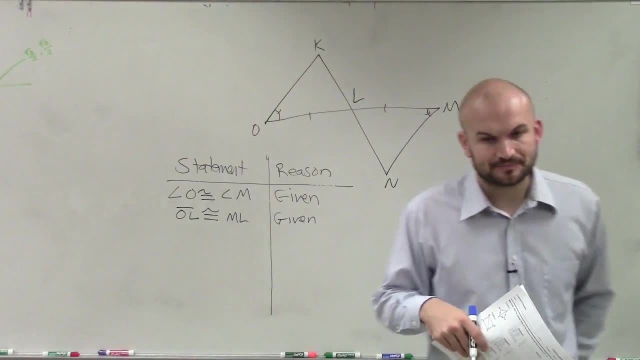 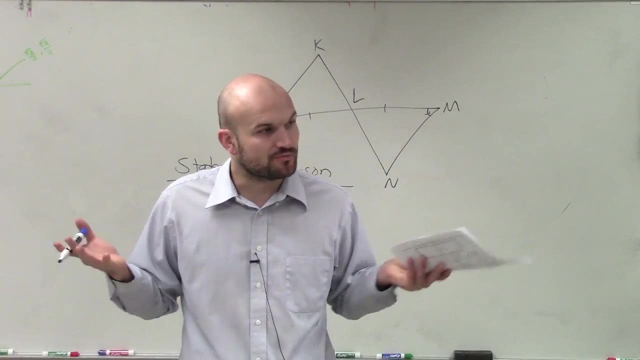 So the next thing that we want to be able to do is look at what else can we prove, Because remember, ladies and gentlemen, when we talked about our congruencies, if we want to be able to prove that things are congruent, 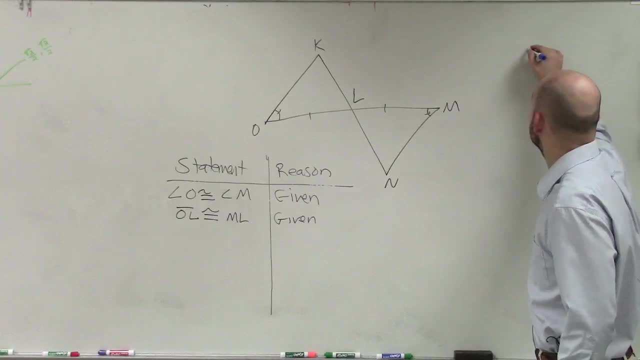 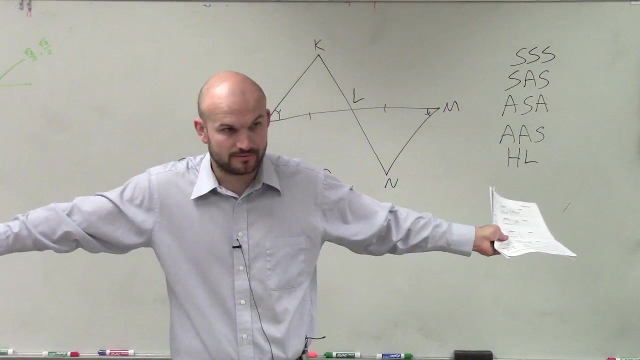 there's only so many congruent statements. We talked about side Side, Side Side, Angle Side, Angle Side, Angle Angle, Angle Side And hl. Those are the only ways we can show that two things are congruent. 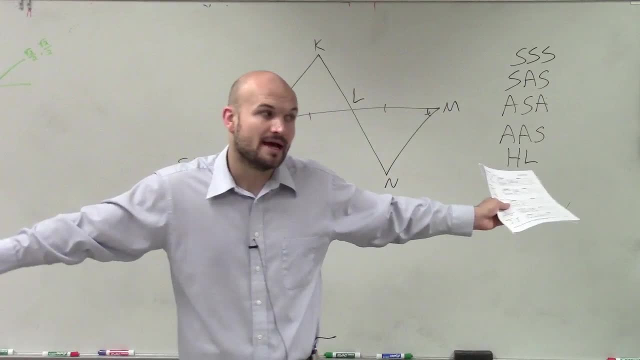 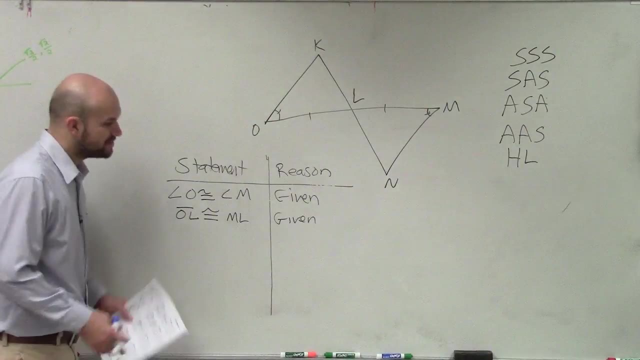 Would everybody agree Angle angle angle is not one And angle side side is not one, unless it is hl, meaning we have a 90 degree angle. So what we need to do is let's look at some possibilities of things that we can prove. 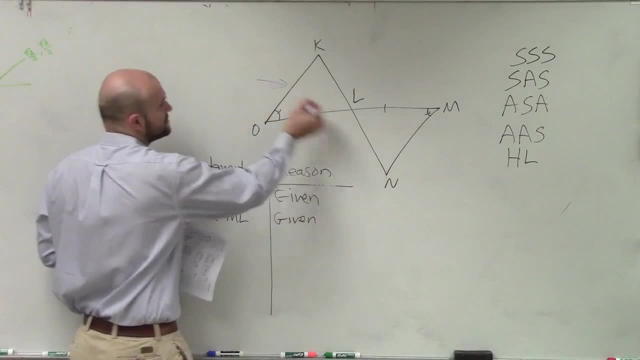 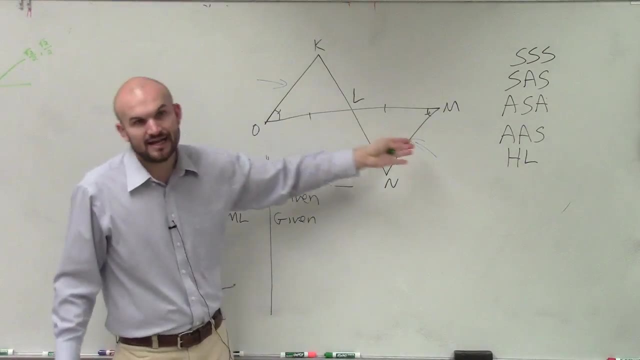 All right, We could look at. Can we prove that these two sides are equal? Because if we can prove these two sides are equal, we have side angle, side Right. But is there any theorem or anything else you guys know? 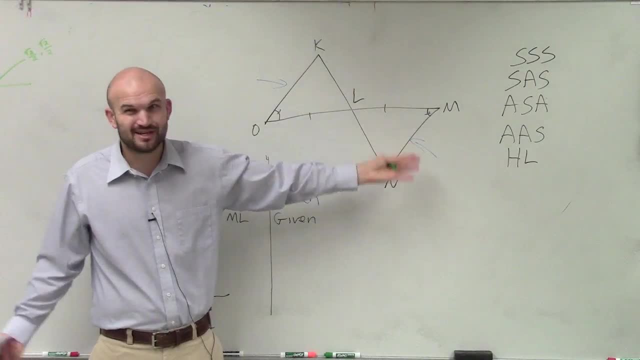 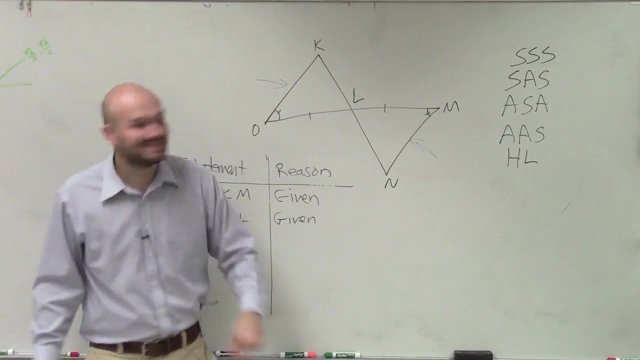 any reason that you can show that these are equal. They look equal, But is there anything you guys know of that we could show that those would be equal for, Yes, Asia Vertical angles, Yes, yes, that's where we're next. 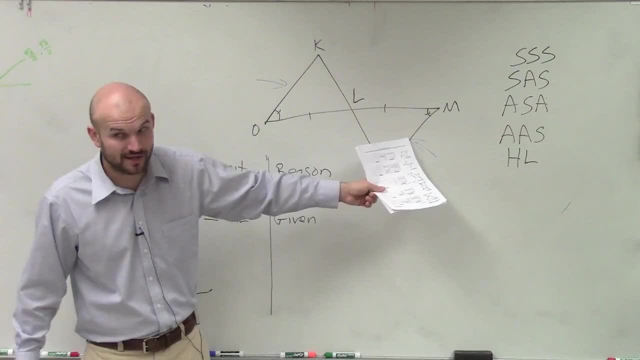 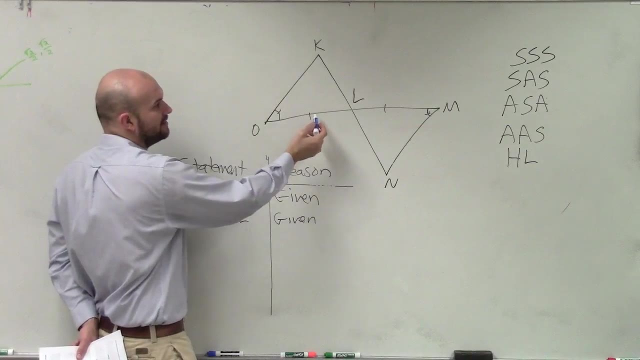 But yeah, we see that these aren't going to be equal. They're not going to be equal because vertical angles. But we'll get to your point exactly where you're at, So then we look at all right, another one. So we can't do side angle side. 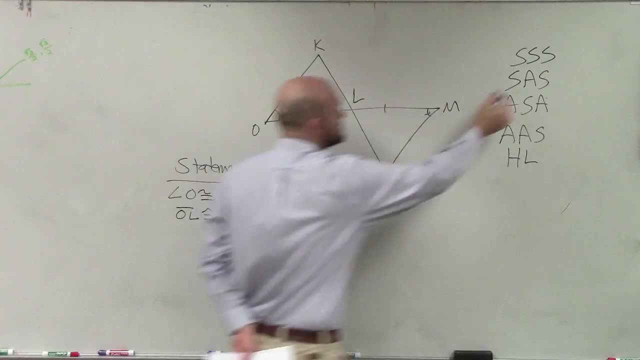 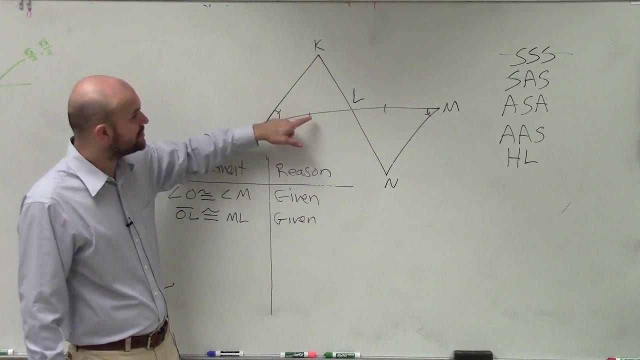 If we can't prove that side then we can't do side side side. So pretty much these congruency statements are out of the question. If I had to do angle angle side, that means obviously I'd have to show that these two angles are. 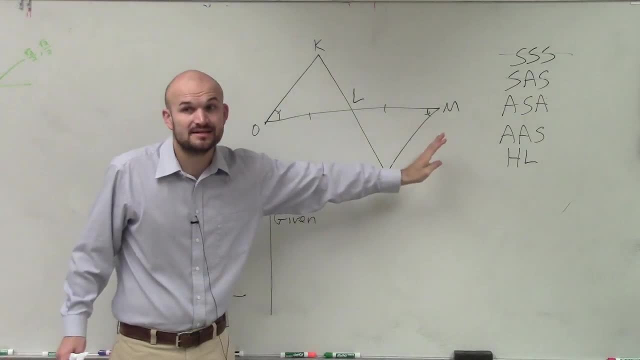 equal to each other. Well, if we knew that these were parallel lines, we could show that these are alternate interior angles. But these two lines are not parallel. At least it's not given to us that they're parallel, So we can't prove that. 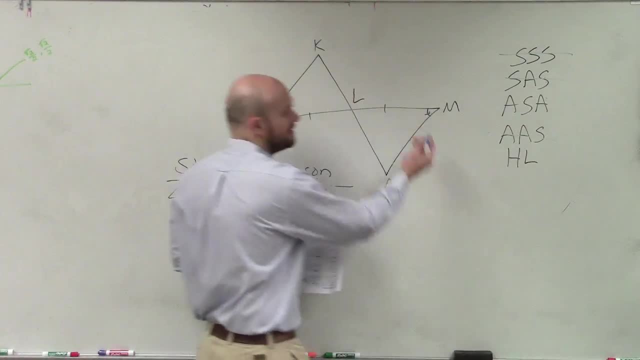 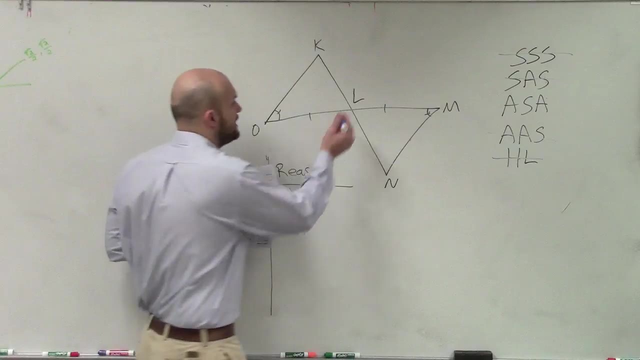 We can't assume them, So angle, angle side- is not going to work. We know there's no right angle, So HL is not going to work. So the only thing we can think about is angle side. angle meaning we have to show that these two angles are. 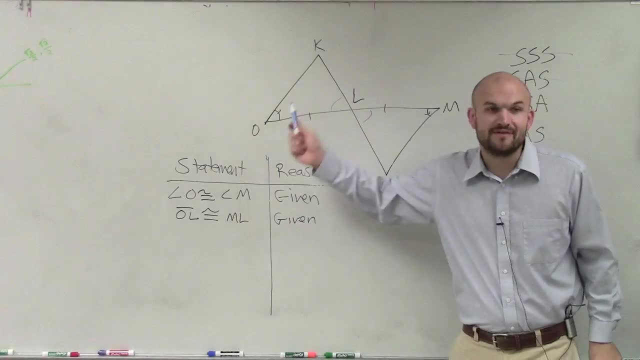 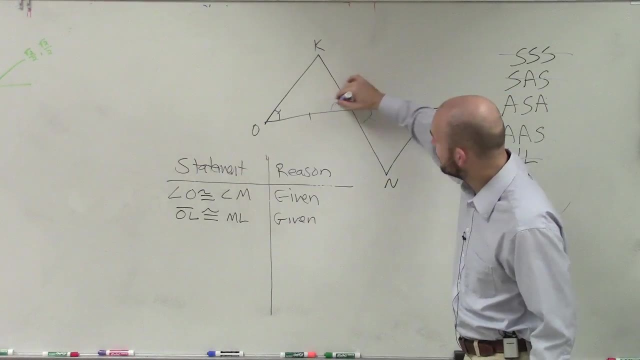 congruent. If we can show that those two angles are congruent, we have angle side angle. So, Blake, what Asia said is: well, those are vertical angles And we know that vertical angles are congruent. So the next thing, what I would say is: 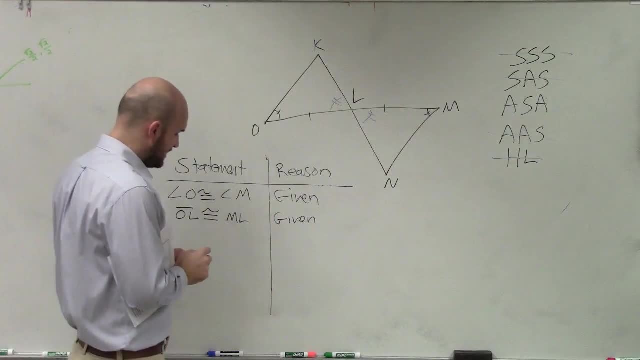 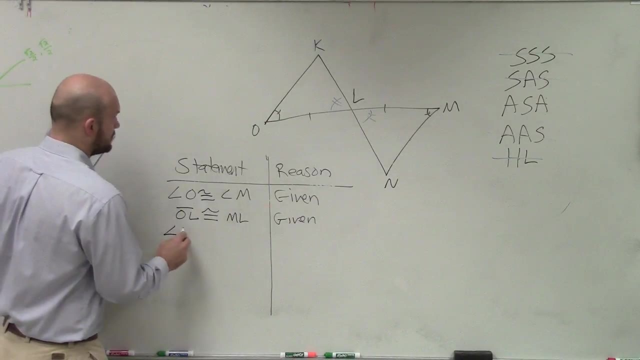 now notice. since these angles are shared, I'm going to use three letters to label these angles. Don't call it angle L and angle L. So what I'm going to do is I'm going to say angle. I'm going to start at my one angle here.